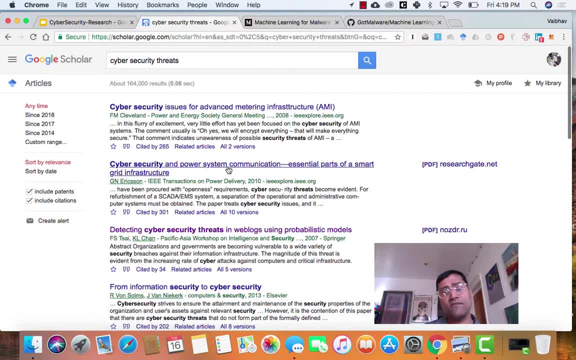 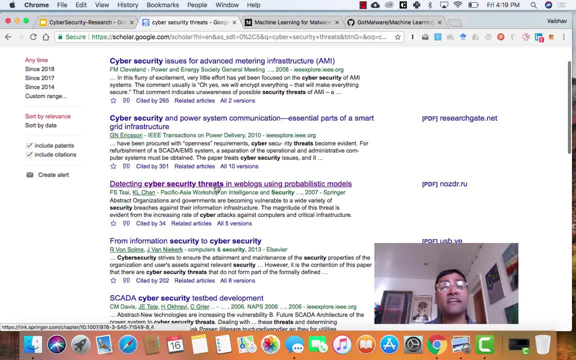 The first one is about advanced metering infrastructure. The second one is about power system communication. The third one, which is interesting, is about cybersecurity threats in weblogs. The fourth one is about information security to cybersecurity, so on and so forth. So I'm curious and I click. 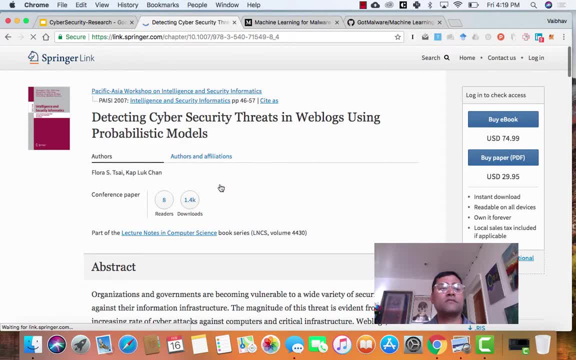 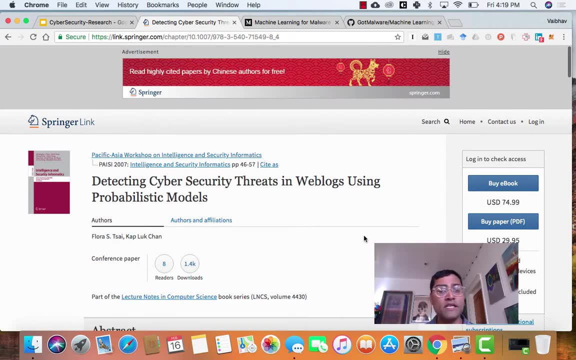 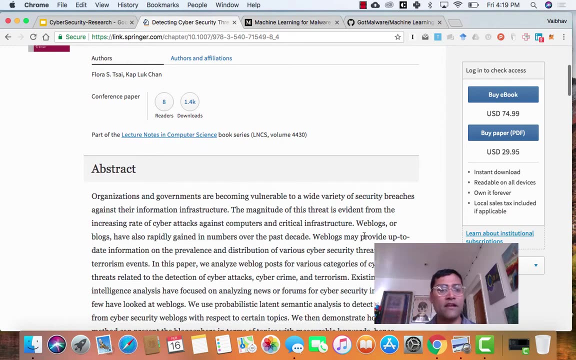 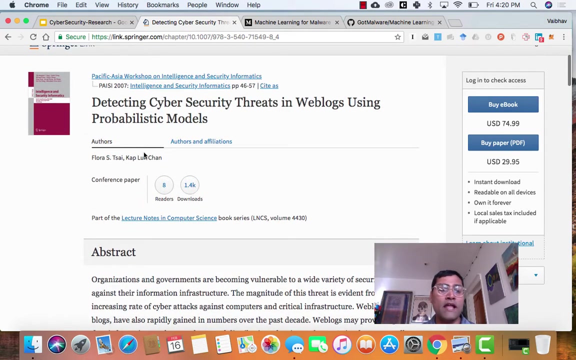 on the third link. It's about weblogs and using machine learning and probabilistic models to figure out if a particular website has been hacked or not. So this paper would go a lot in detail about it. This is a paid paper so I can't go in and buy, but I encourage you to go and look for. 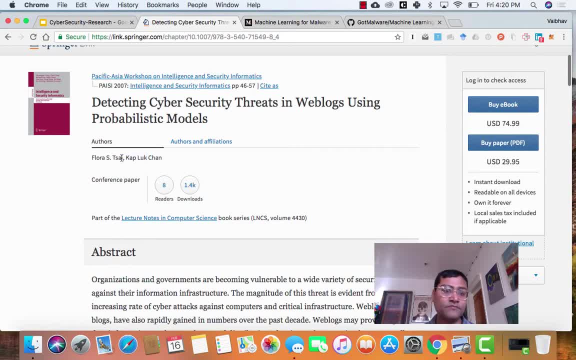 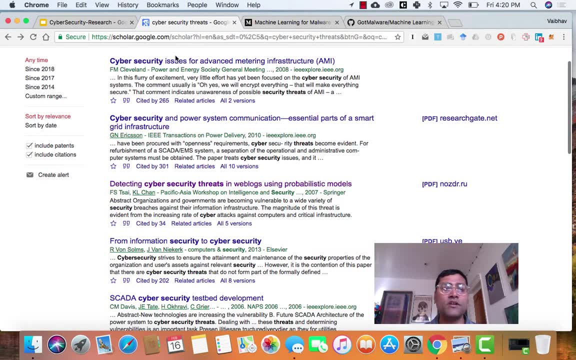 the authors of these papers. In this case, it's this author, Flora, and I'm going to search for any research they have done. So in this particular case, I'm just going to say googlecom And I'm going to search for Googlecom. 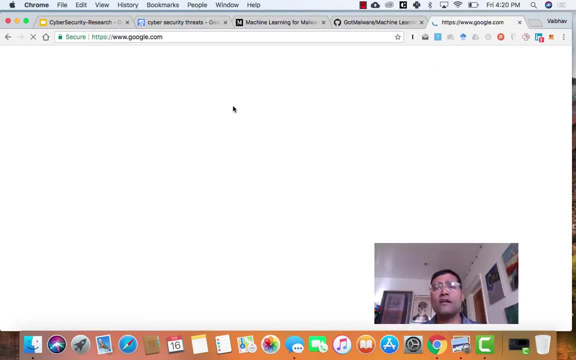 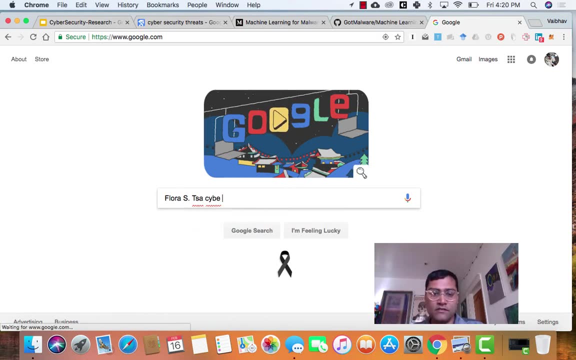 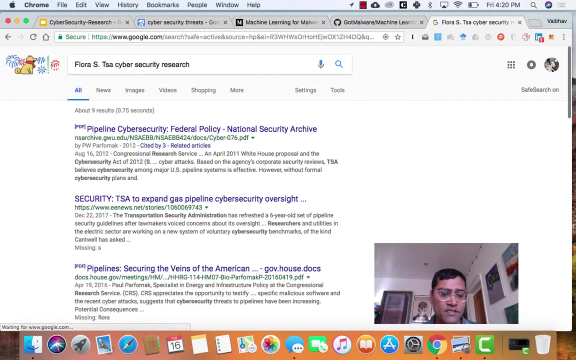 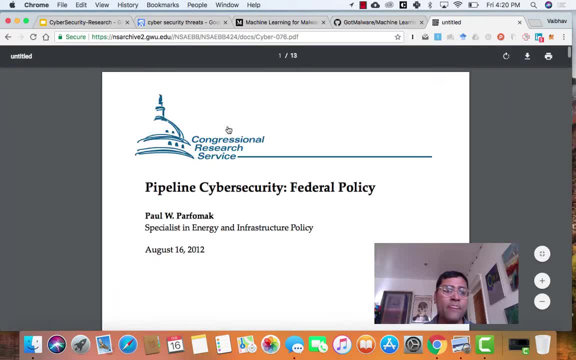 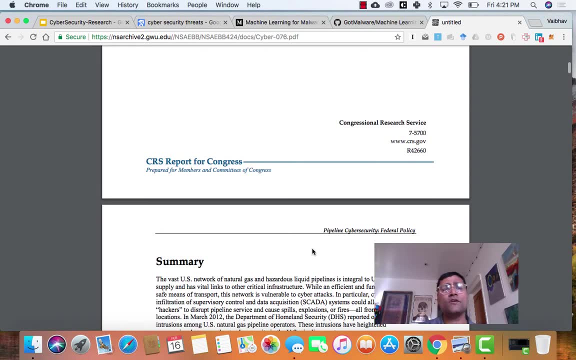 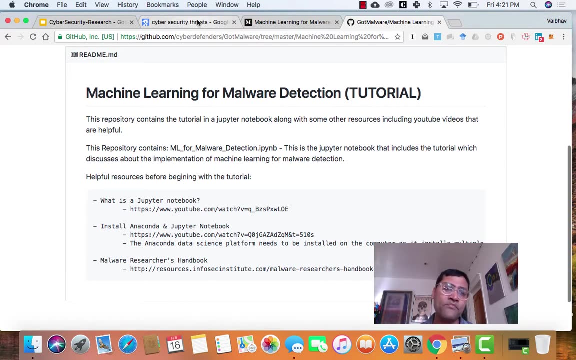 the top one is about pipeline and cybersecurity, And we can go through federal policy around it and so on and so forth. I would encourage you to kind of go down this rabbit hole and look for a few interesting topics in cybersecurity. I won't spend too much time on it. 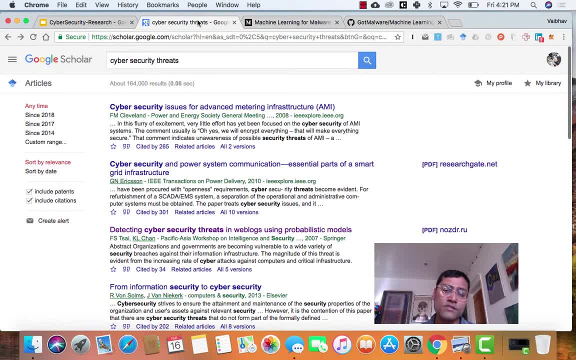 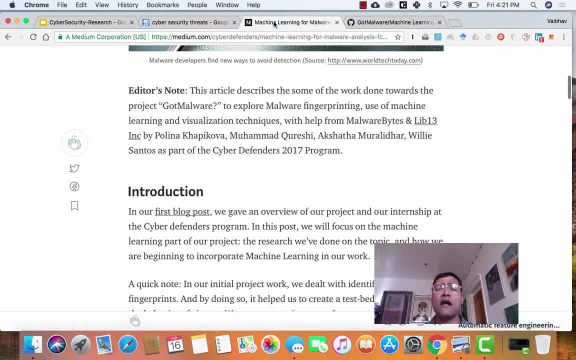 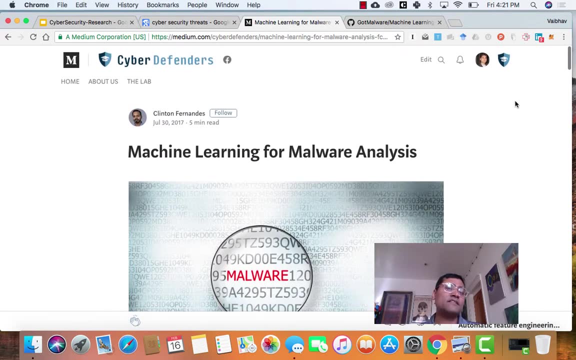 Second thing we want to do on this module for the course is talk a little bit about advanced topics. So the particular advanced topic I would like you to know more about is machine learning in cybersecurity. So cyber defenders has a great blog, So we have a good article on machine learning for malware analysis. 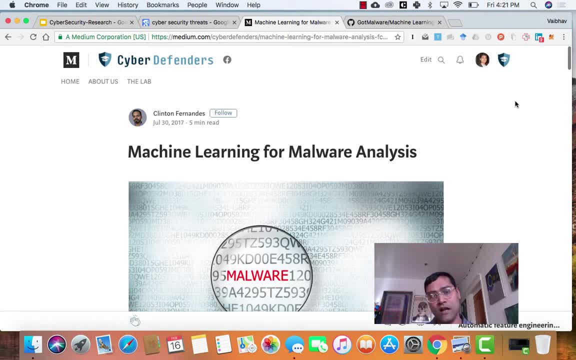 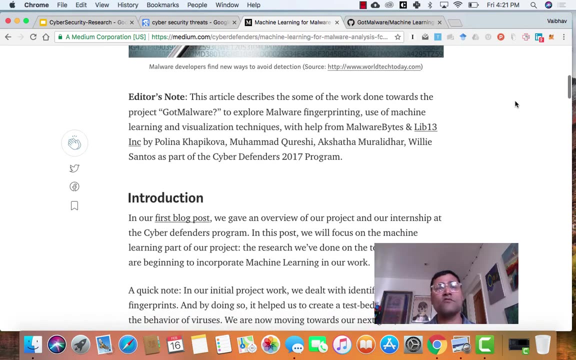 I highly encourage you guys to read this article. The link for this particular article is in the course notes. Machine learning for malware analysis is all about finding patterns, in particular malware. So malwares are viruses which cause harm to a malware And, in particular, malware is a virus. 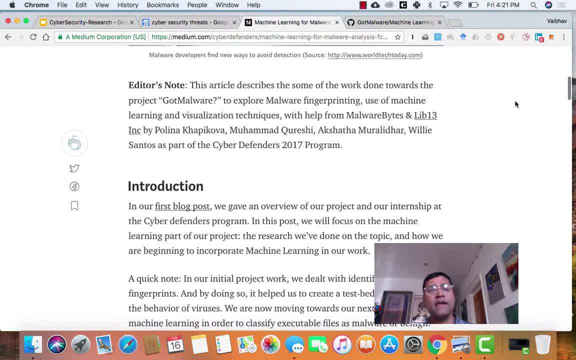 So malware is a virus. So malware is a virus. So malware is a virus. But malware is not necessarily a virus And malware might cause harm to the machine. In previous sections of this course, we looked at how different tools can assist you in doing. 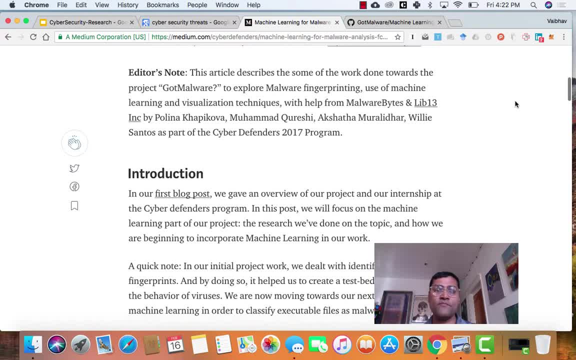 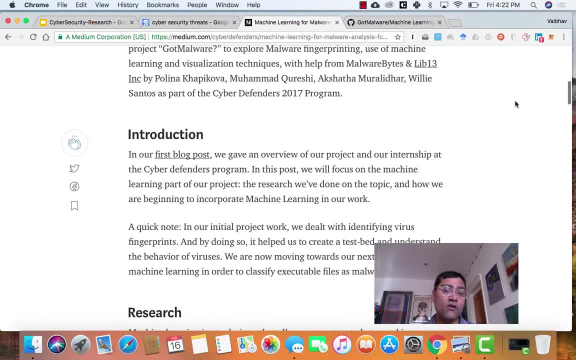 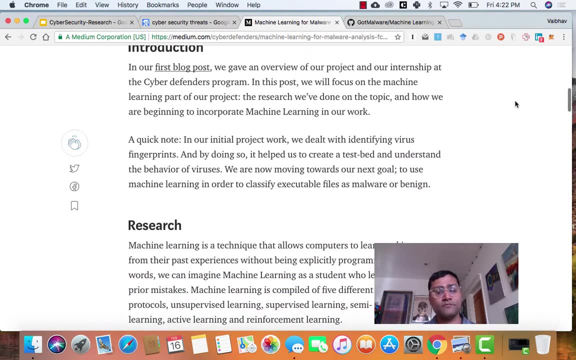 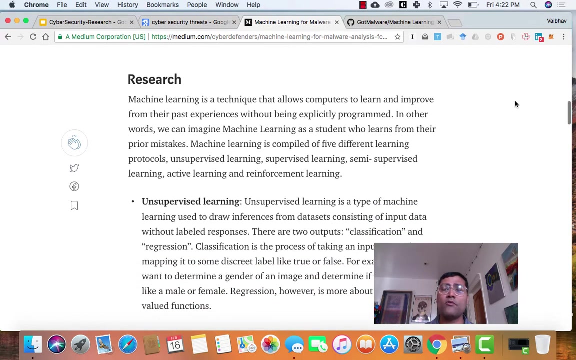 exploits or finding exploits in existing software. So this one helps you to figure out a pattern in particular malwares. So this blog post is very detailed. It is about machine learning for various types of Android viruses. Yes, So a link from this blog post is to our github website. 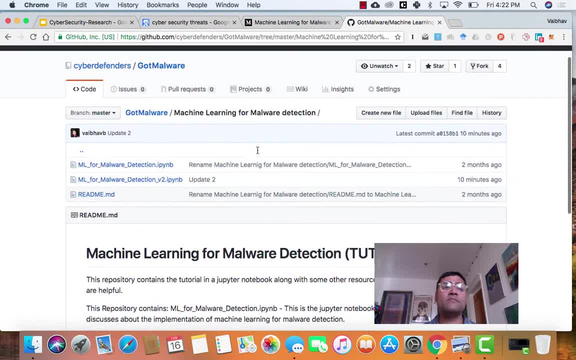 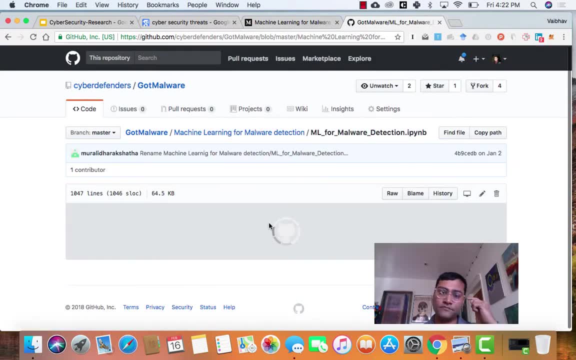 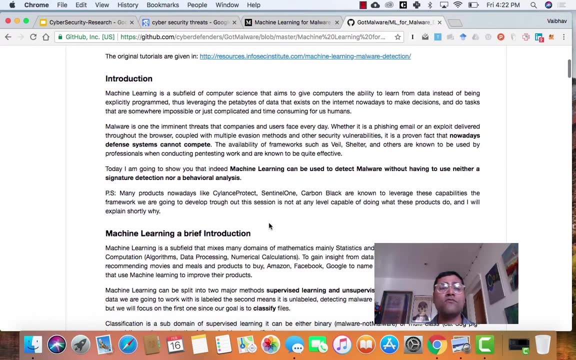 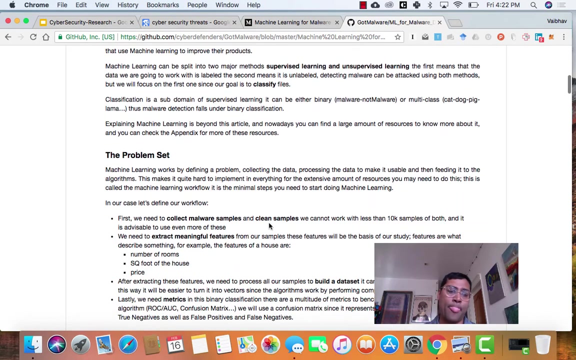 Which I'm going to click. next, The website has code for doing machine learning in Python. So in this particular Repository you will find Code to follow on and do machine learning on Android viruses. So in this particular case, I'm just going to give you an overview of what this python script is about. 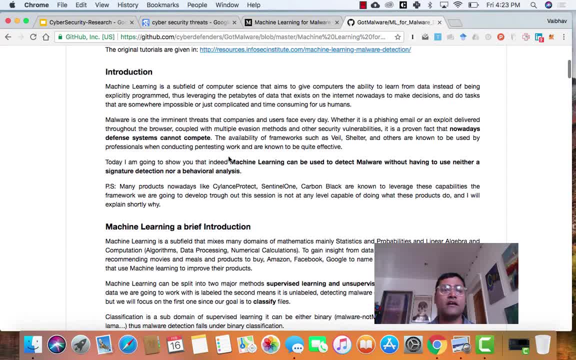 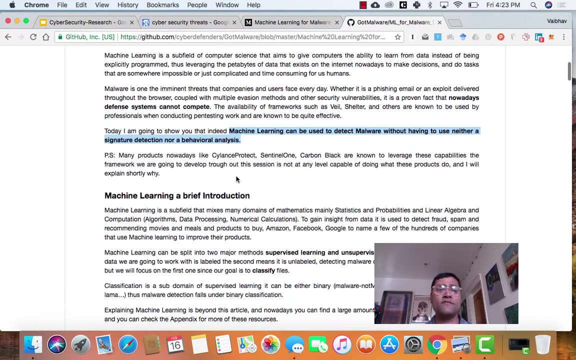 It gives an introduction to machine learning. in this particular case, machine learning can be used to detect malware Without having signature or behavior analysis done. again, those are both advanced topics but just giving you a sense of what kind of Behavior analysis happens on on on malwares before you can figure out if that particular software 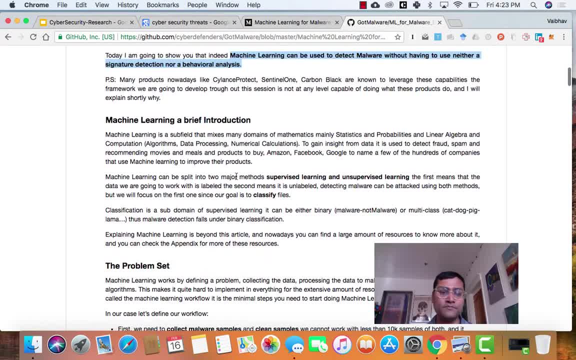 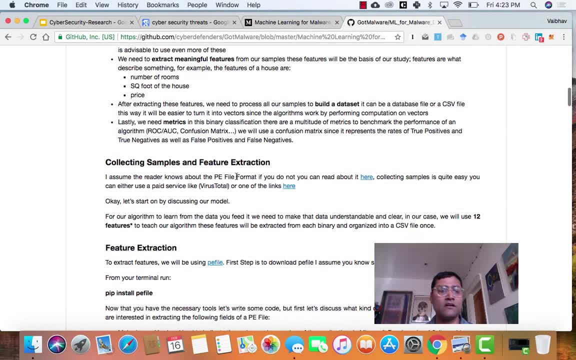 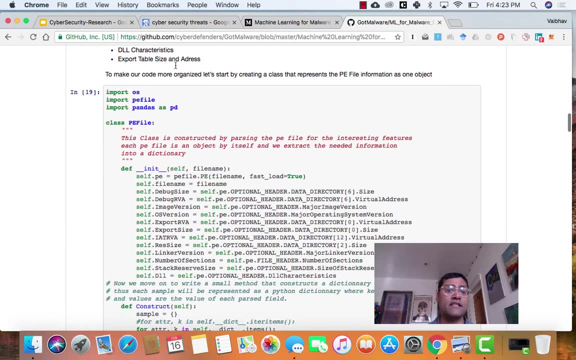 Is a malware or a functioning piece of software. In this particular case, what we're trying to do is build a data set based on Certain features in the software. so the software goes through finding features in PE files And and it goes through using some machine learning and data. 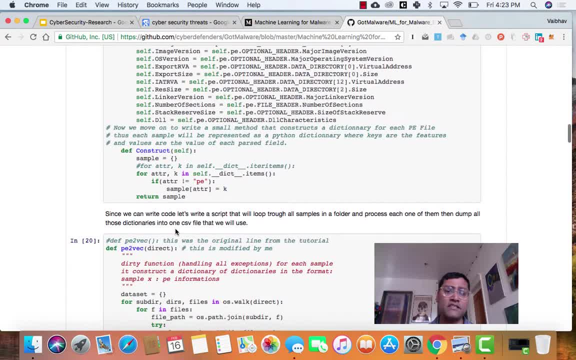 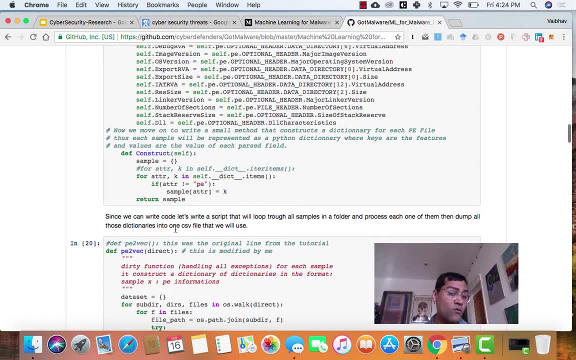 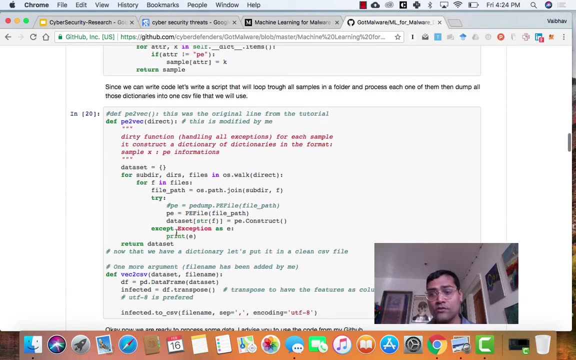 Analysis tools. if you follow through this particular python program, Which is written in a jupyter notebook, you will get a good sense of what it is Like. we do not require you to to follow through this, But I highly encourage you to read and if you, if you do have the time to follow through.